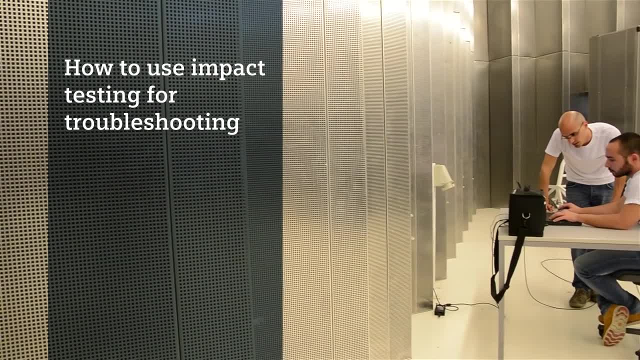 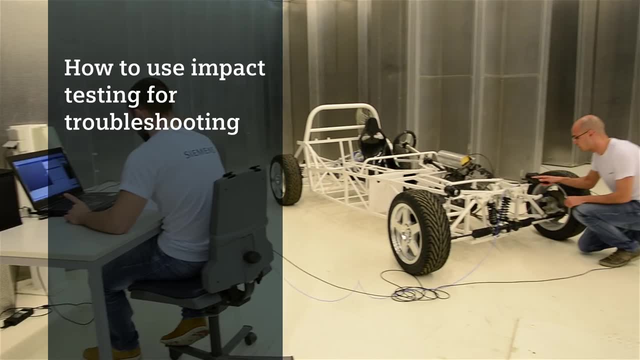 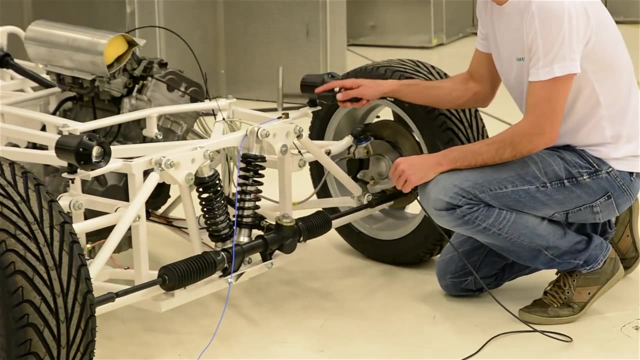 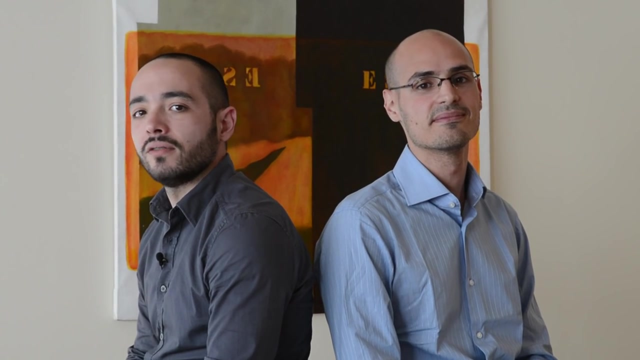 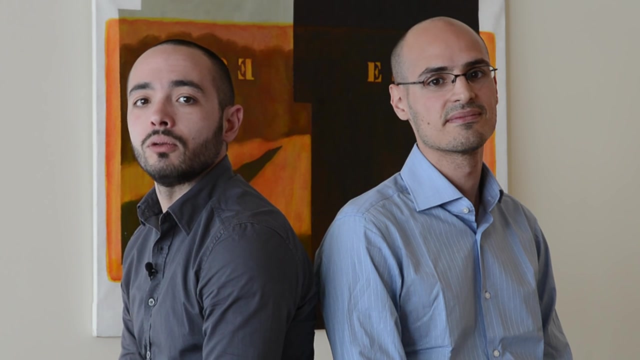 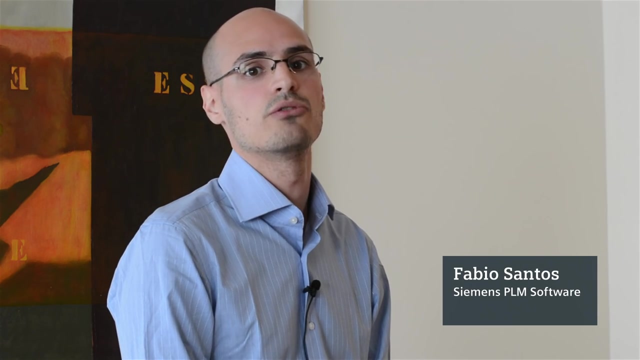 Hi, we are Simona and Fabio from Siemens PLM Software. Many engineers face problems of excessive operational vibrations on a daily basis. Today, we would like to show you how to resolve these issues using impact testing. Unwanted vibrations during your system's operation can be attributed to two main sources. They can either result from operational force, as generated by your system's rotating components, or they can be a consequence of resonance, Especially in the second case. so when dealing with resonances, impact testing will help you to localize and resolve your system's unwanted vibration issues. 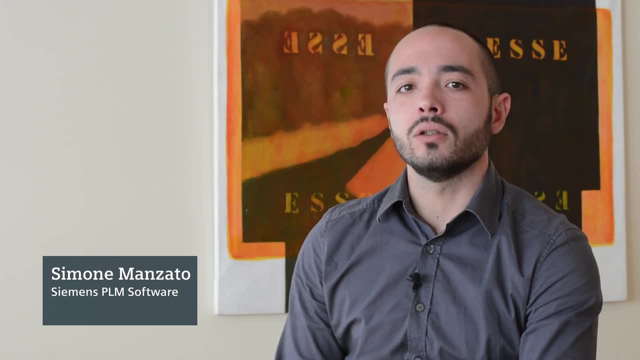 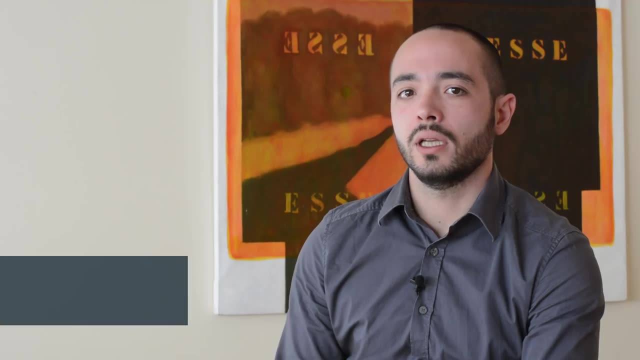 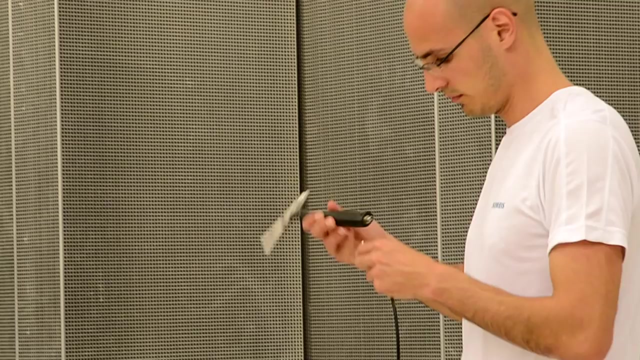 Impact testing is quick and easy and delivers clear and intuitive output. Moreover, the Siemens approach to impact testing only requires limited instrumentation: A few sensors, for example: accelerometer to measure the system's response, An impact hammer instrumented with a full cell to excite the structure and measure this. 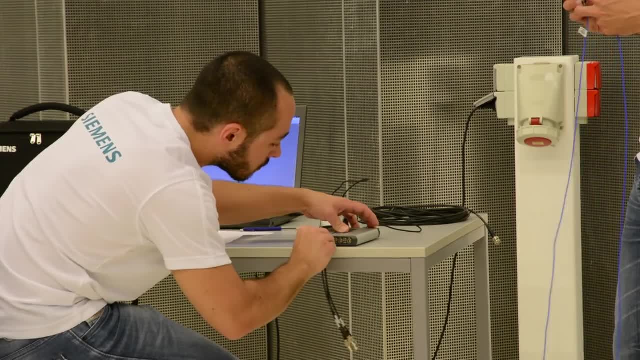 excitation. A SCADA 6S to acquire the system's vibration. A SCADA 6S to acquire the system's vibration. A SCADA 6S to acquire the signal. A SCADA 6S to acquire the signal. 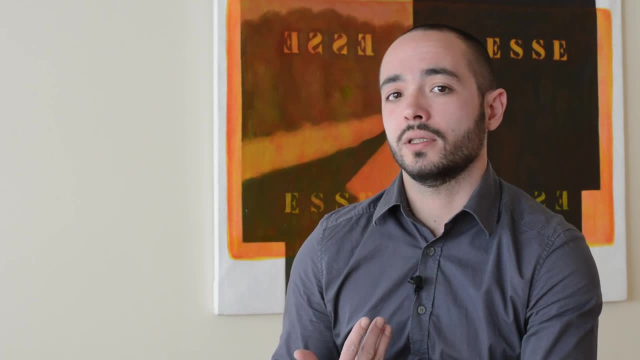 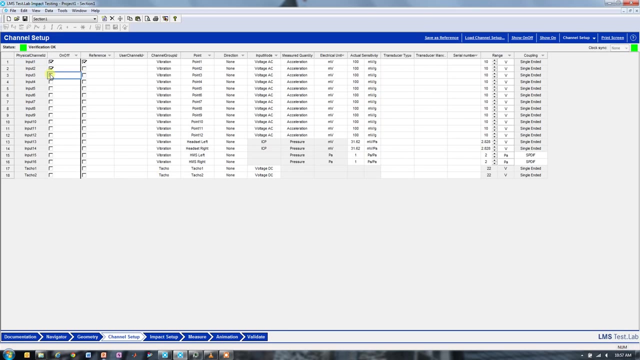 And the laptop running LMS TestLab software to manage the process. First, your measurement needs to be defined in the channel setup. As you can see, the setup allows you to specify all of the relevant characteristics. You can describe your transducer's location, its direction and its measured quantity. and 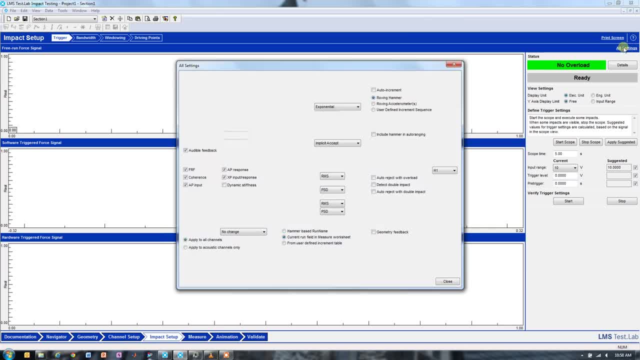 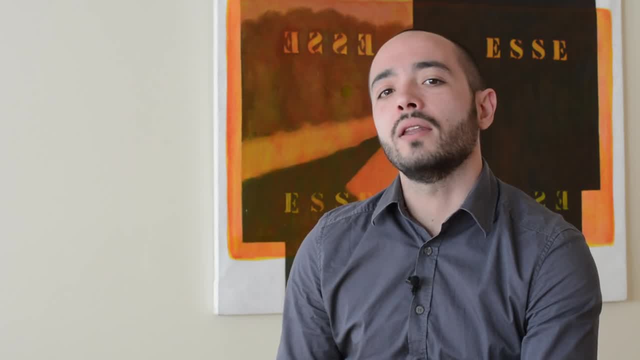 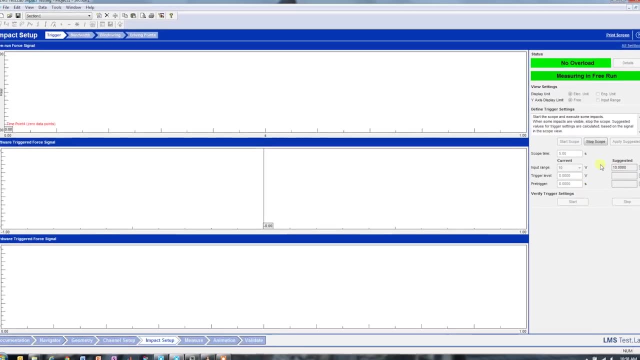 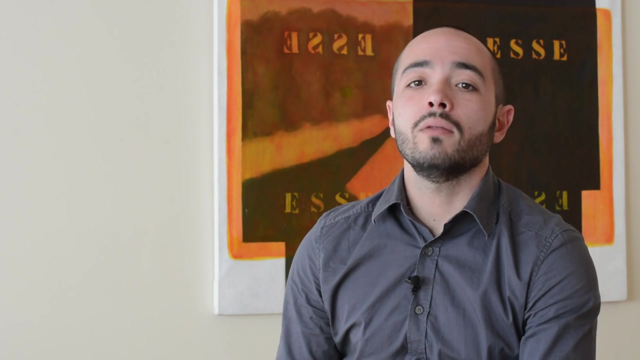 sensitivity. Next, you will need to define your impact hammer's so-called trigger level. When you use it to hit the structure a few times, LMS TestLab will derive a unique set of trigger parameters all by itself. Finally, your measurement's bandwidth needs to be checked. 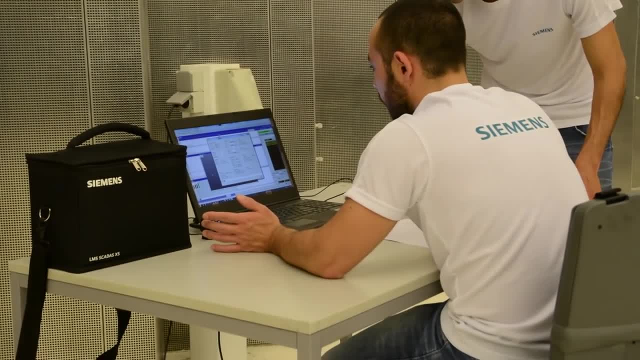 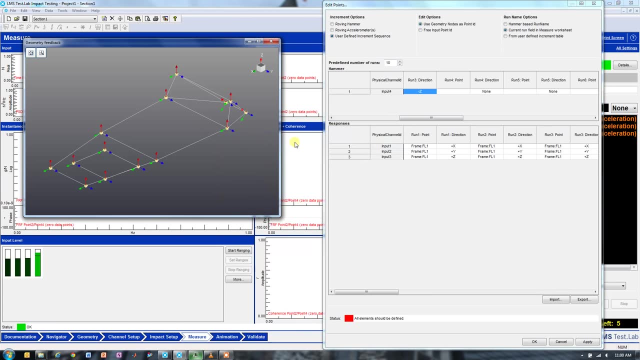 The bandwidth you are looking for depends on the frequency, range of interest and instrumentation you choose. To make things even simpler, the software will assist you in making the right selection of tools. For instance, it will reflect the accuracy of your choice of hammer tips in its results.